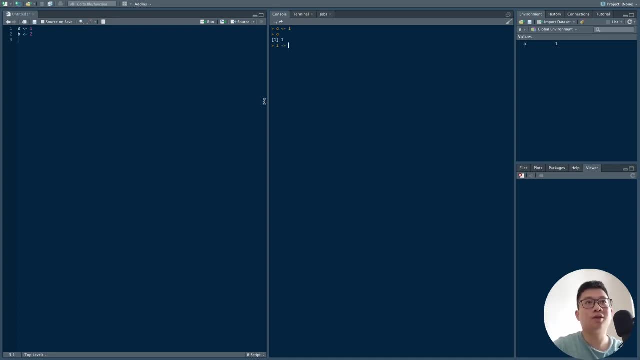 do a right-hand, do a dash, right-hand A, So A will also be number 1, right. So we seldom actually use a right-hand assignment. We always use a left-hand assignment, And then if you actually want to assign it with using the equal sign, it's fine as well, But most of the time we actually 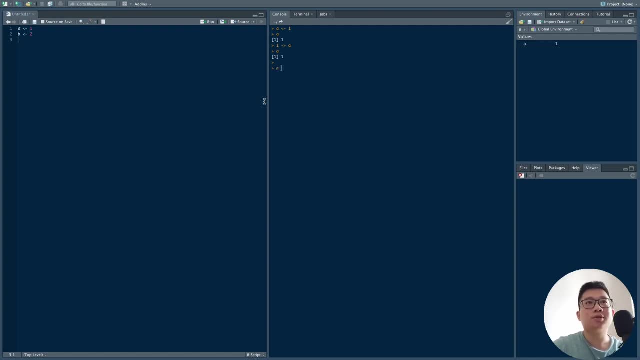 use this arrow symbol, So A equals to 1.. We also create the assignment of 1 to the variable A right. So if you look into your RStudio over here, we're actually going to do all the examples on the console And then this one itself is a script. 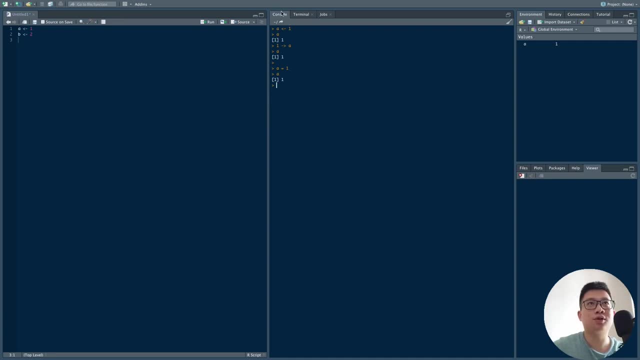 So how do you actually differentiate between these two? is that over here you can see a console, which is this environment, And then for script, usually you have a run button over here. So if we recap what we did in the previous tutorial, for script-wise, we can't, we won't see. 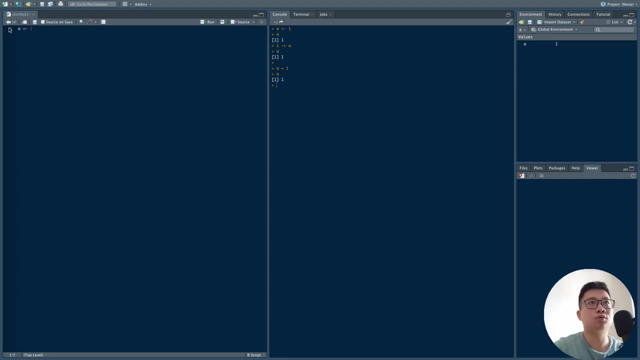 an immediate response when we actually type in our code. So if we click on enter it will just move on to the second line, As opposed to over here. when we actually do it on a console, we get a straight response over here. So A itself is equals to 1. And over. 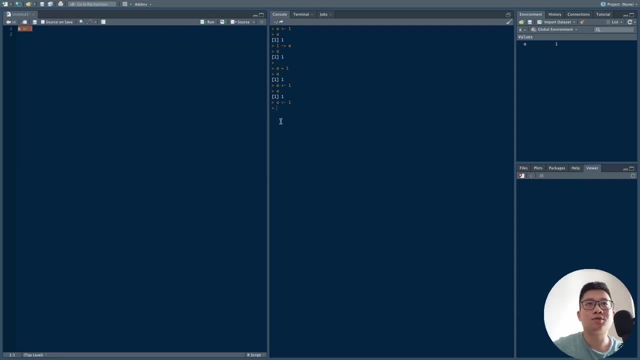 here I have to highlight the whole thing and then click on run in order for this to run right. So this is just something you have to take note when we go through the example later. So next up, let's spend some time talking about print statements. So if you go through any, 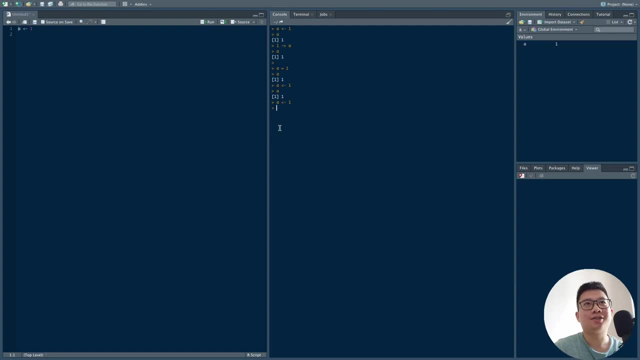 any coding tutorial, it will actually tell you all. you know, the first thing you ever do is to print the hello world statement. we are going to do the same. So, in terms of printing, it's quite straightforward. we do a print, we type in, print And then, over here, we put in a brackets and then we type in. 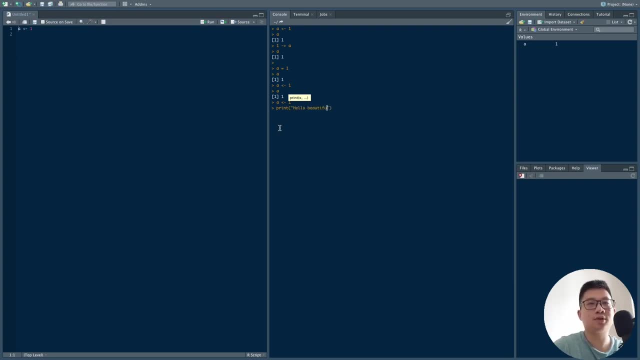 hello, beautiful people of the internet. And then you will get printed up straight away. So print statements are quite important. So let's say, if you actually want to check if whatever functions that you have applied onto a specific variable actually works, we will actually use a print statement inside the function to see. 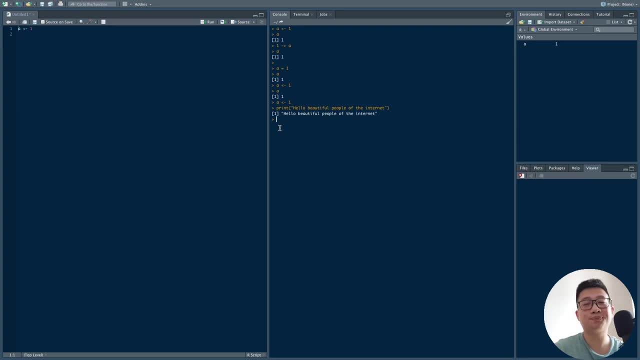 if it actually works. So we often see ourselves doing print statements, But then it's important when we actually push the program, when we push the program to production, it's important that we actually get rid of the print statements, Otherwise it will actually show up at the 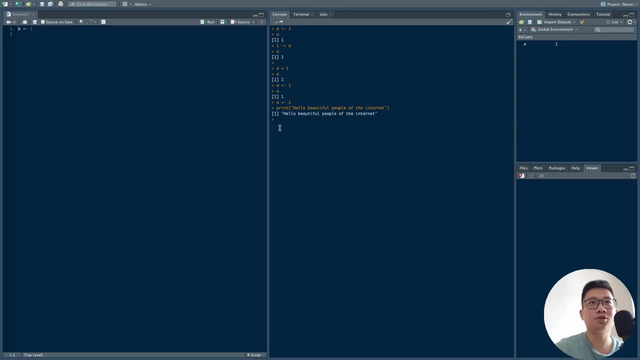 log when we actually look through it. So this is something that you have to take note. So something you may have noticed is that when we actually do the print statement, we actually put the statement in between two quotations. The reason for that is because 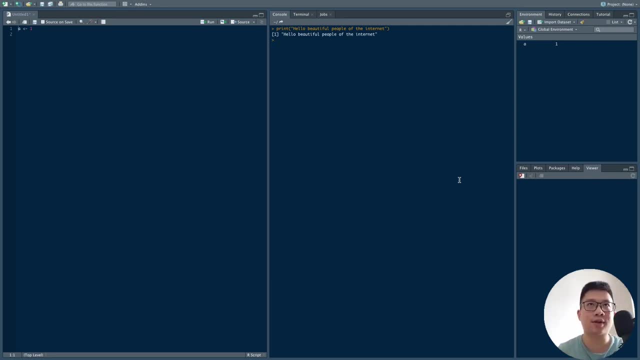 the statements are characters. characters are actually words. So there are different data types that we are going to talk about later. They are the characters, they are numerics, they are logicals like true, false and na, And then there are complex numbers of words. 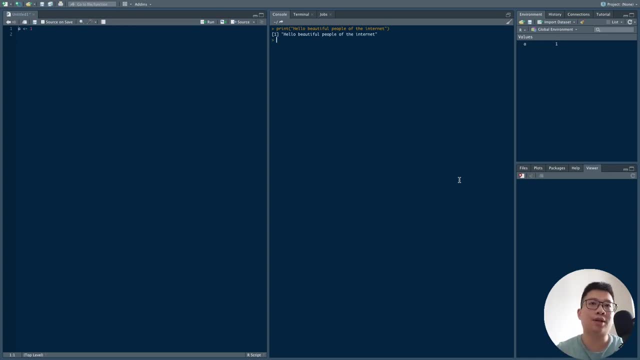 numbers, there are also raw data. So raw data are like bytes, something that a computer will actually understand. So when we actually do a print statement, for example for a number, you actually don't have to put that number in between a quotation. So if we do a print, 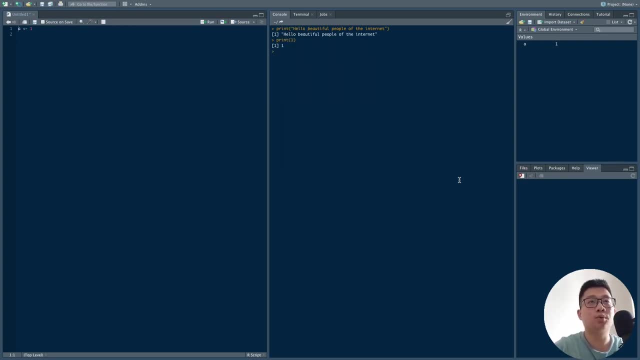 of one, it will actually show up as one, So we don't have to put it as a quotation. But notice, when I actually put it in between the quotations, what we see here is actually completely different from what we see on top. So what happened here when you actually put something in between a quotation? 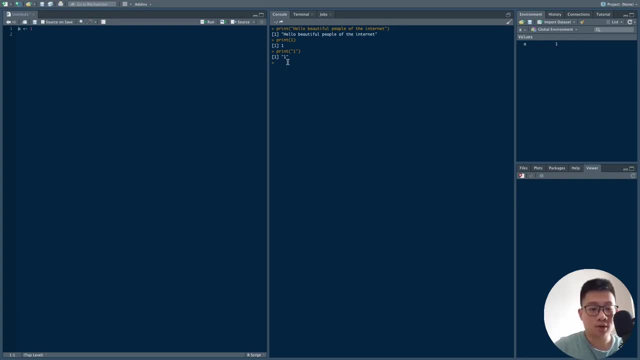 is that it will be converted to a character. So let's say we do a type of Type of is a way for us to actually find out the type of the variable that was assigned. So over here let's say we do a type of one. in between quotations You see that it's actually character. But then if we actually 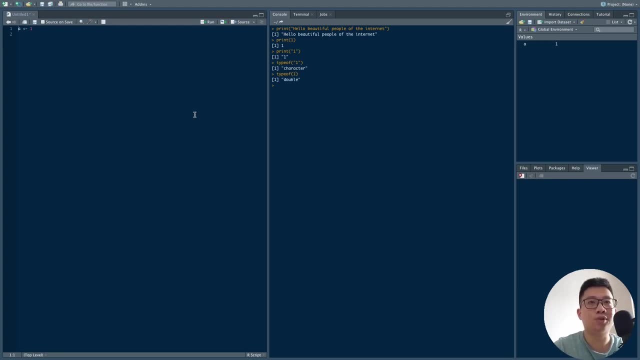 remove the double quotation, it will actually be a character. So let's say we do a type of one in between quotations, it will be a double. So a double is a form of numeric value And most of the time for R they will actually classify any numerics as a double. So when you actually do 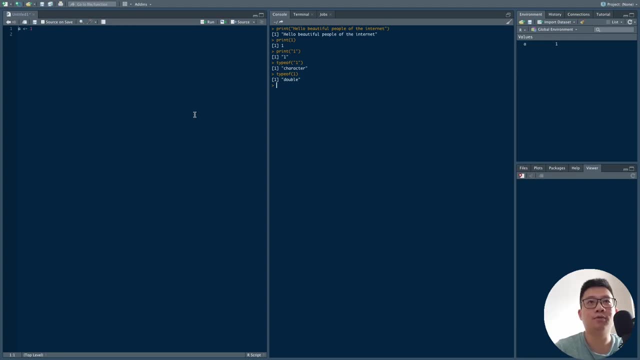 assignment of any form of data. even for logical data like true and false, it's important that you don't put them in between quotations, Otherwise you'll be converted to a character, And if it's a character you can't add anything. So if I do one plus character, 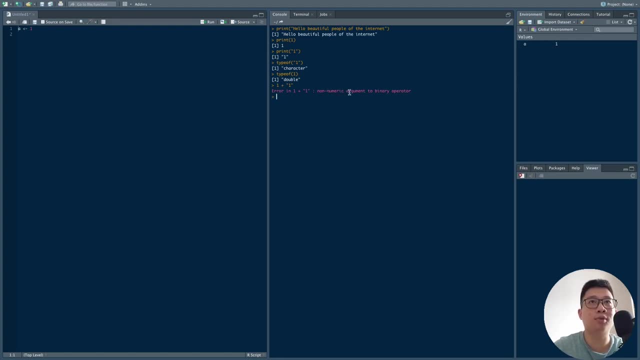 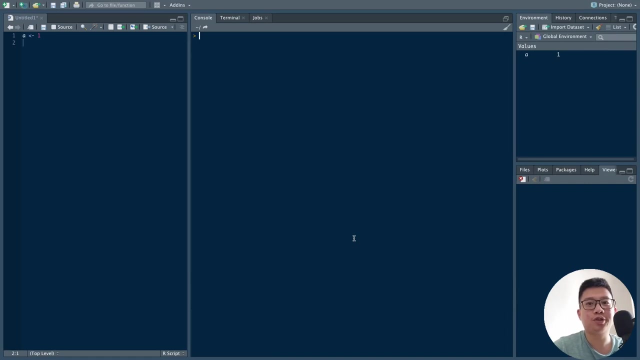 you get an error message to say there's a non-numeric argument to binary operators. This itself is a character. You can't add a character with a numeric. It just doesn't work. So this is something that you have to take note. So next up we are going to talk about addition, subtraction. 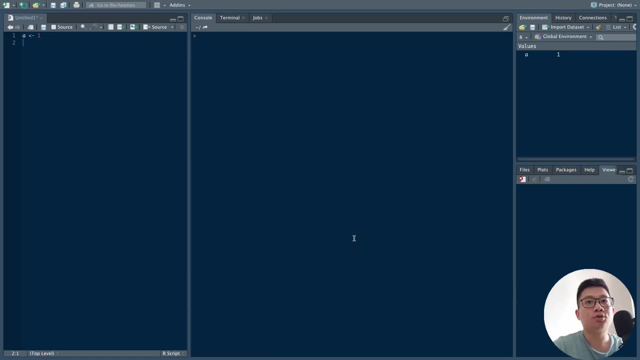 multiplications, division and also remainder. So when you actually do addition, subtraction and all these mathematical functions, it's actually quite straightforward. So you can just, for example, if I do print 1 plus 1, I just do that and it will show up as 2.. Same applies for a number. So 1 minus 1. 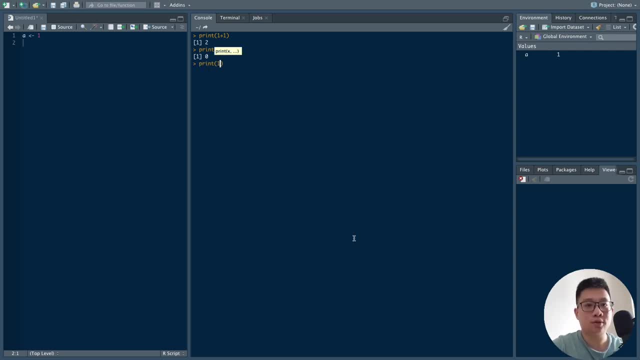 will be 0. And then multiplication is just using the star symbol, which is shift 8.. And then we do 9.. For example, it will be 1 times 9, will be 9.. And then, lastly, we'll be doing division, which is: 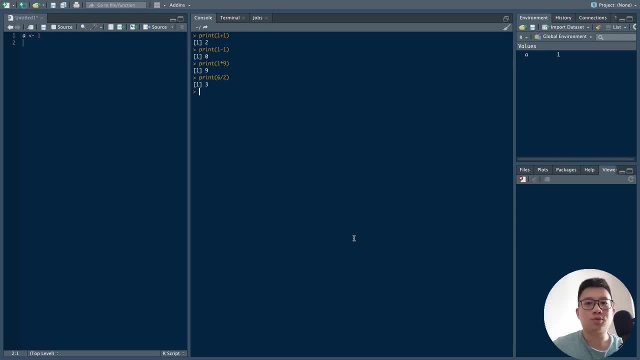 let's say 6 divided by 2 will be 3.. So the next one we're going to talk about is remainder. So to identify the remainder of the division, for example, let's say if we do 6 divided by 4, the 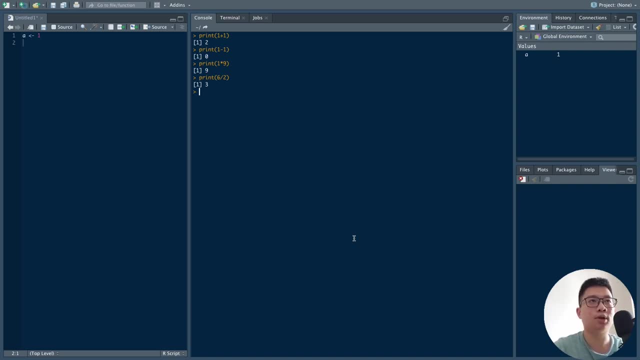 remainder is 2.. So how do we actually identify this remainder? So we're actually going to use this symbol, which is a double percentage sign. So if we do that, we actually get a remainder of 2.. So when do we actually see ourselves using this? 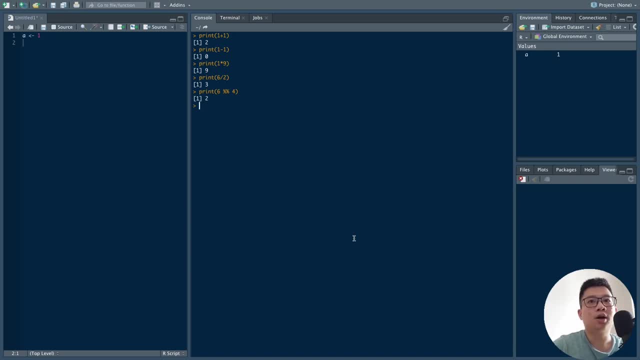 double percentage sign thing. It's when we actually want to identify, to see if this variable is even or odd number. right, I think some of the time when we actually do some coding problem, they will actually ask you: how do you actually prove that this variable is even or odd? So one way is to. 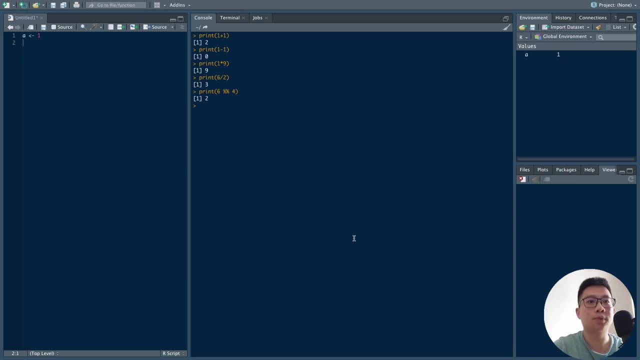 use. this is divisible sign. So for example, let's say, if I sign the variable gets to be 8 and then I assign B to B. one right itself is a even number, one b itself is odd number. so what i can, what i can do, is i can. 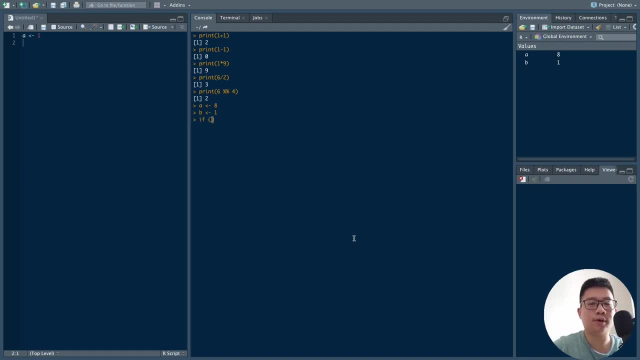 say if i'll talk about if else statement, conditional statement and in a later tutorial. but this is just to prove that, um, we can actually know if a variable is an odd or even number, so a itself if it's, uh, divisible by two. so when divisible is something that's divisible by the 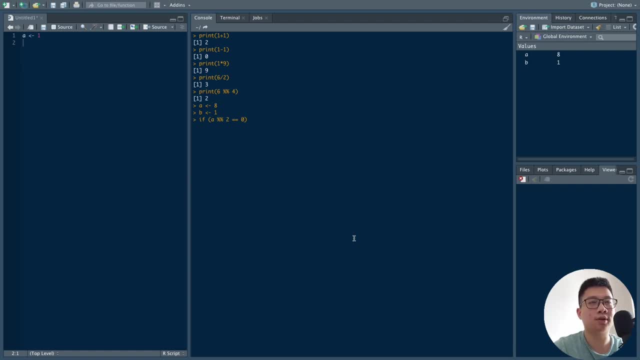 number, it actually generates a zero remainder. all right, there's something: if you take note and do a print, uh, if it's a, a will be print event number, else print odd. so you can see that a itself is an even number because it's actually generate. it generates a. 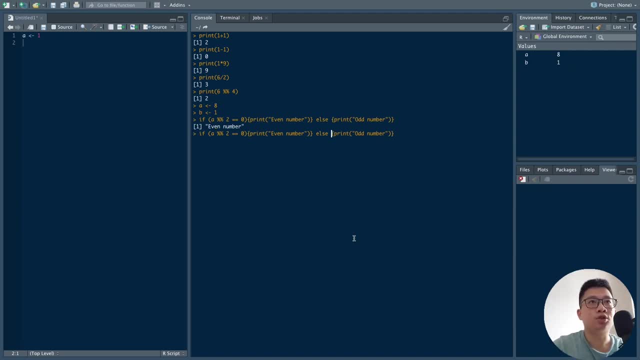 zero remainder. but then how do we actually check that it's a odd number? we can actually do the same with b. so b is a one. one there by two will generate remainder. so we'll say it's odd number. so as simple as that. and then you may have noticed that i actually use the double equal sign. so when 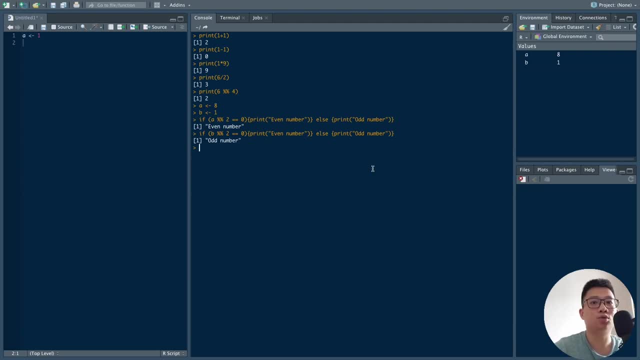 the double equal signs means that it's actually directly equal to the double equal sign. so when the double equal signs means that it's actually equals to a, something that you actually want to test out. so let's say, if um, a is equals to test, and then we want to check if it's actually exactly to that, to that character. so if, if a is, 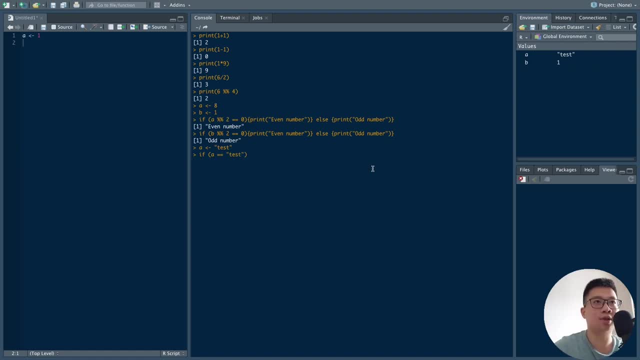 equals to test, right, because it's actually. we want to see if it's actually exactly the same as same as this character. so if that's the case print, actually we don't have to do this. uh, let's see if i close this this one second. so what we can do is we can do a. we already know a is test, so a is equal to test. 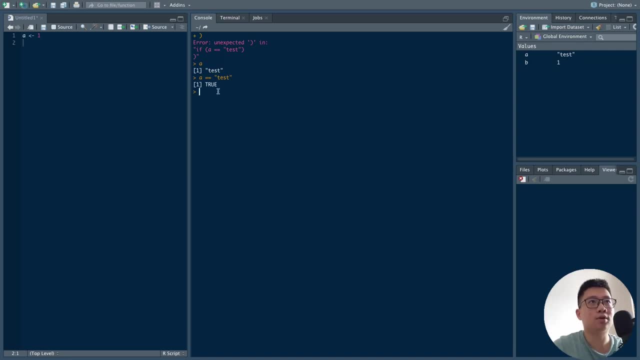 which will then return a boolean. that is true, right? so how do we know if it's the opposite of a double equal is not equal, so how do we actually assign a not equal is, to use an exclamation mark- equal, let's say, if it's a cake, for example, which will then return a boolean. that is true, right so? 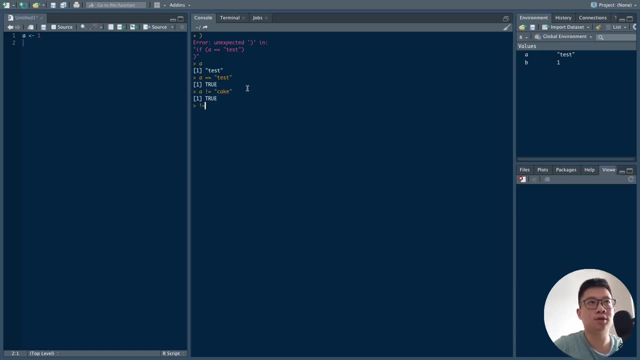 a is not equal to cake, so not equal is an exclamation mark and an equal sign, and then equal is a double equal sign. so the reason why we don't use a single equal sign is because a single equal sign is used for assignment of variable right. so a equals to one is assigning one to a right, but a 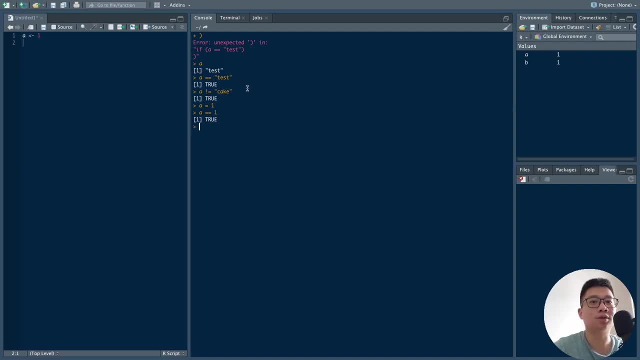 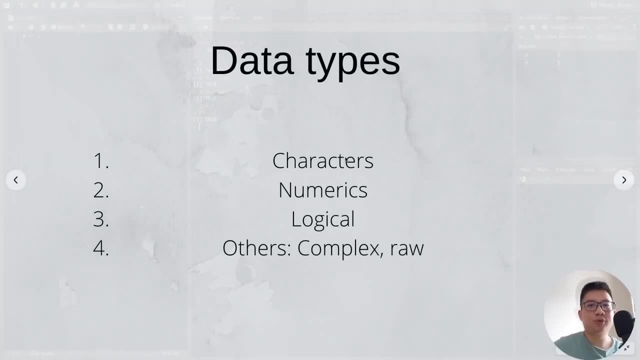 double equals to one is checking the equality to see if a is actually equals to one, and then it returns true. when it is, uh is equals to one. so next up, we're actually going to talk about data types. so there are five types of data: characters, numerics, logical and also complex and raw data. right, so for character is actually 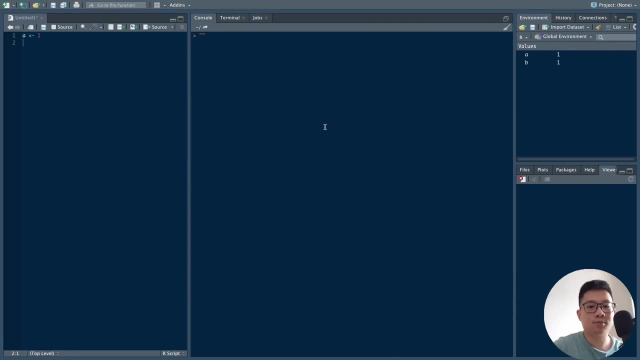 quite simple as well. i say: anything that's assigned between a double quotations will be a character. so let's say, if i assign a to be a test, and then how do we actually check for the type- the character type, i mean the data type- of this variable is to use this type of function. 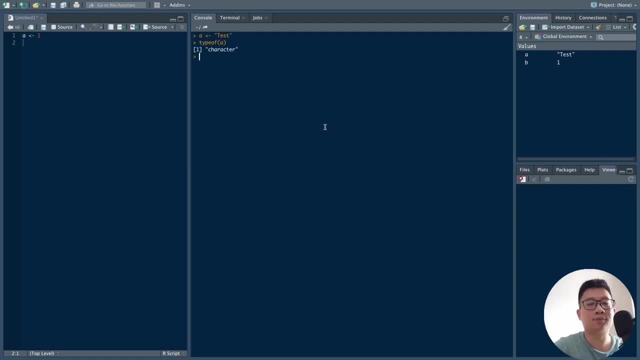 and then we type in a and then you'll tell us that it's a character, right? so next up is numerics. so, numerics, there are a few types. they are integers, they are decimals, but most of them are actually- uh, belongs to this double class, this class called double in r. so, for example, let's see if i do a type of one, two, three, so that's what i'm dealing with here- let's say two bar, then if i'm going to talk about a dashing or denominator, this comes from dashing or the learning definition of a format set. and first is it serves to dafür hло b government. so winner nap a key number like not a key number. take in werd a key number. 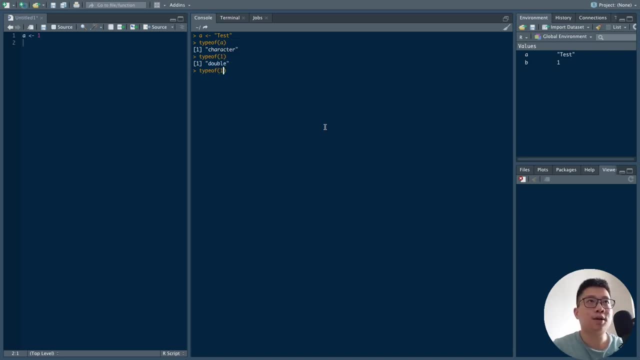 it will be a double. if I do a type of 1.1, it will also be a double right, a double itself. it will always be converted as a double, regardless of whatever non-numeric value it is. so next up is logical. so for logical, there are three types. they are true, force and na. so let's. 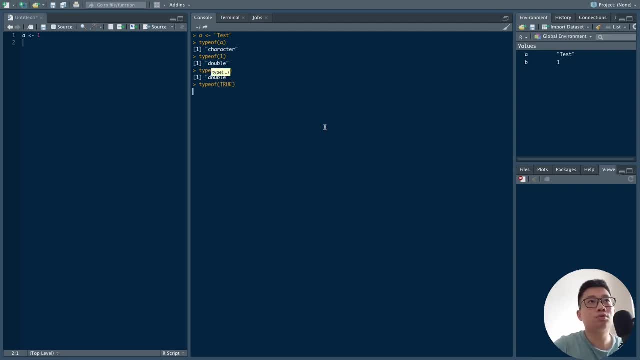 say, if you do type of do true, it's a logical, and then force it's also logical. same applies for na right. so logical values are something that you will often use in conditional statements: if and else right. because if and else uses- uh, uses the true and false in order to actually execute. 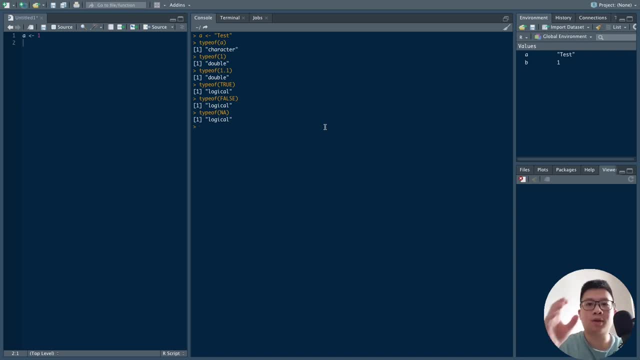 the following lines of code: so if something is equal to something, this one actually returns a true or false statement, then you execute the code. so if it's true, it will execute a code. otherwise you'll actually it will not execute a code unless you have an else statement. then you actually execute that. 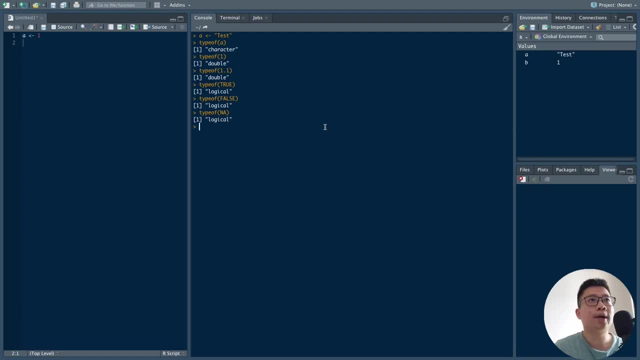 false statement, right, so what else do we have here? so next up is a complex number. so complex number is something that we don't use that often. so, for example, if I do a, assign it to be 1 plus 1i, so it contains this imaginary number. so we do type of a, it will be a complex number. 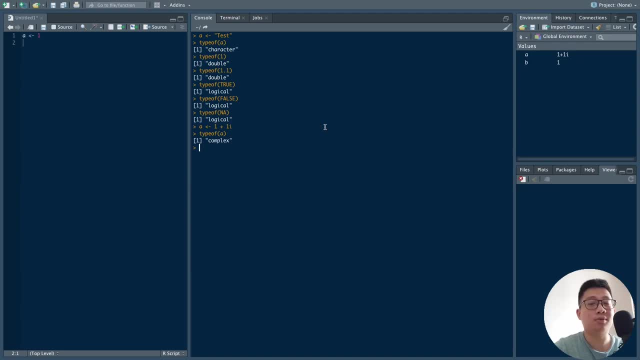 I don't often see myself using this, but maybe, unless you're doing some mathematical calculations, then you'll probably use this complex, uh, this complex data type. so, lastly, is a raw data type. so for raw data type, it's uh, let's say, if I want to actually 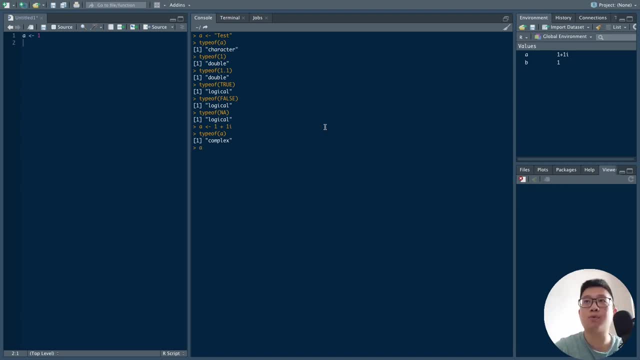 convert something. let's say, if I have a character, once again I'll use the test. oh, let's say I want to convert this character to a raw data type. so raw data type are data type that comes in bytes, right? so let's say, if I'm always char to raw a, so you convert it into. 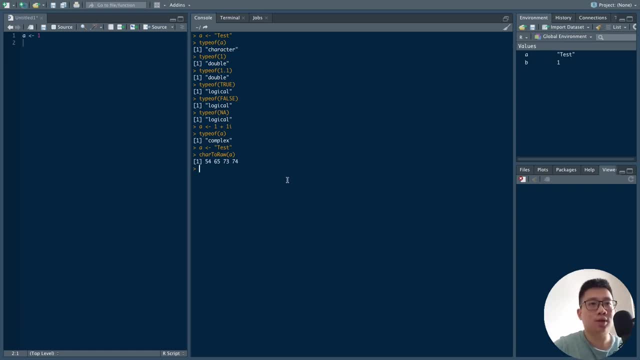 bytes. so if you actually want to convert it to integer, let's say, if I do int to raw, into bits, bytes, if I'm not wrong, into bytes, into beats, bite, Beats- yeah, it's just coin bits. yeah, so you actually convert it into the following: bits Bites, yeah, flowing bytes. 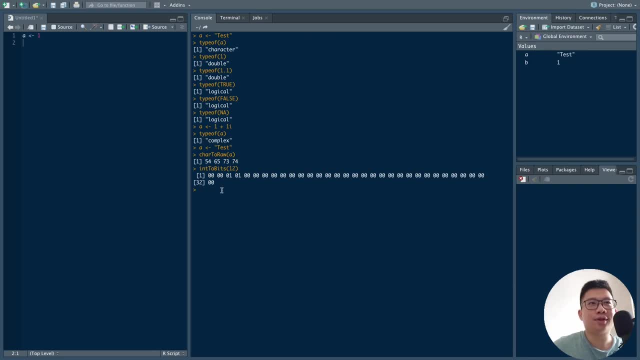 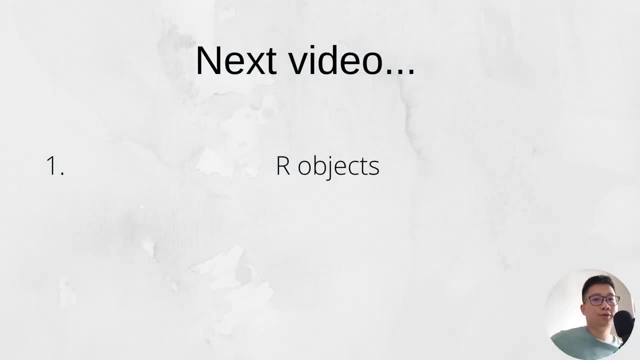 so I don't really see myself using this that often. mainly the three are the characters, numerics and logical. so this is it for this video. in the next video we'll be talking about r objects. so if you have any questions, uh, with regards to this episode, you can actually comment down in the description.